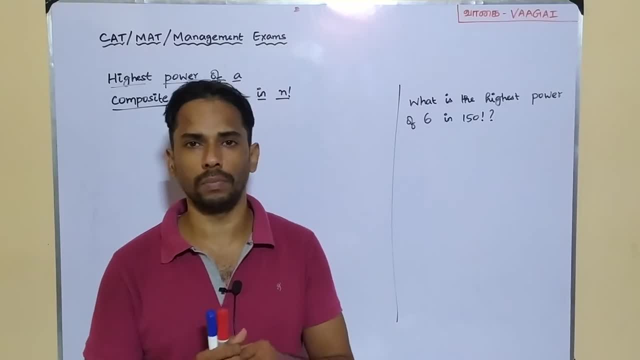 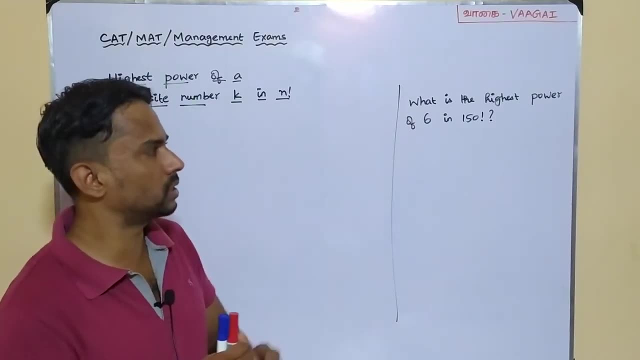 factorial. So in our previous session we saw the very basic concept. We saw also some example: factorial- How can I find the highest power of a composite number there? So that is what we are going to see here and also we have got a problem here. What is the highest power of the number 6? 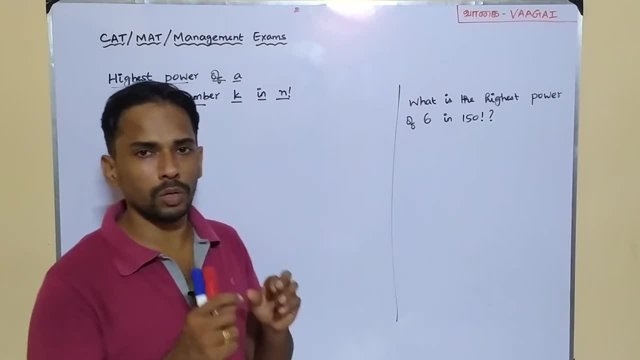 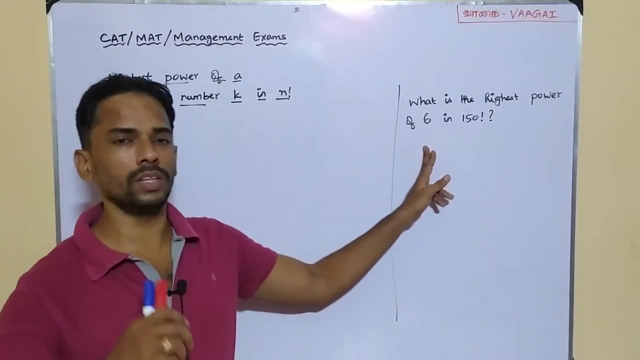 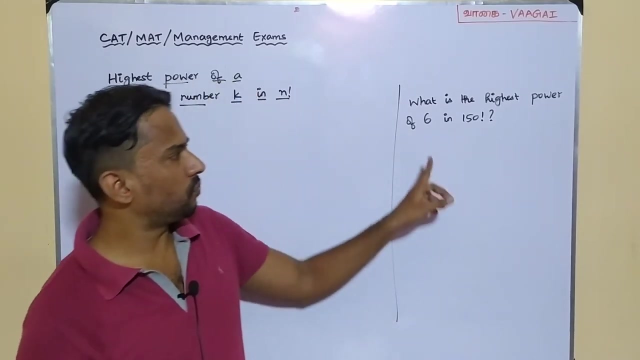 in 150 factorial. So it should be noticed that the number 6 here is not a prime number, It is a composite number, Is it or not? And we are supposed to find the highest power of 6 which we can find here in this 150 factorial or otherwise. I can say: if 6 power x. 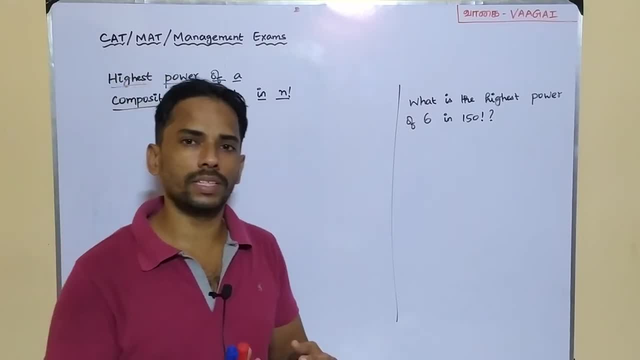 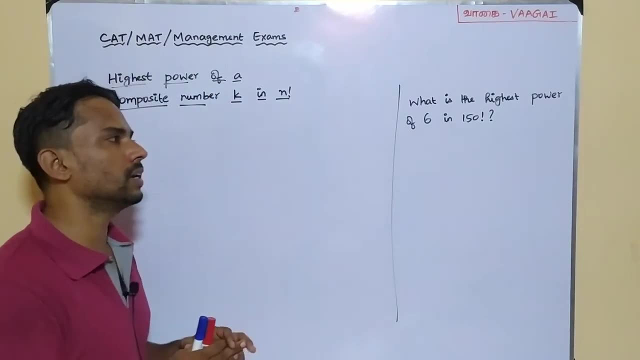 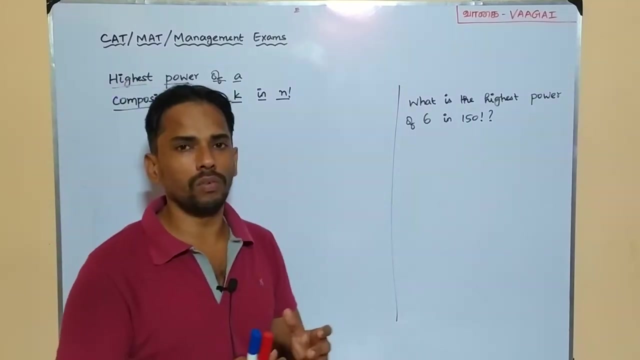 or I can have what 6 power x inside 150 factorial in such a way that my x is the highest number. This is the objective of this session. yes, And we will try to find or learn the concept through this problem itself. So for which, what we need to do, that we will see here. 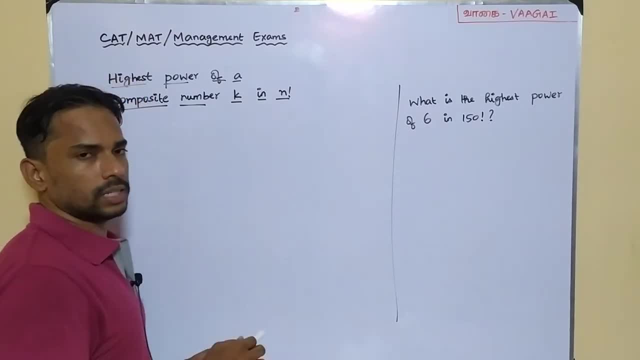 So, as I told, our number here 6, it is a composite number, right? So once we are given a composite number, we must do the same thing. So we are supposed to find the highest power of 6 in 150. 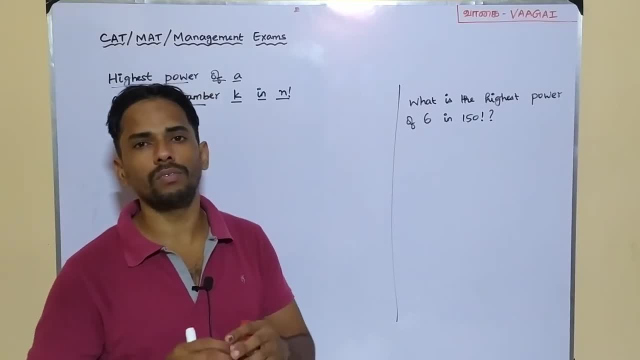 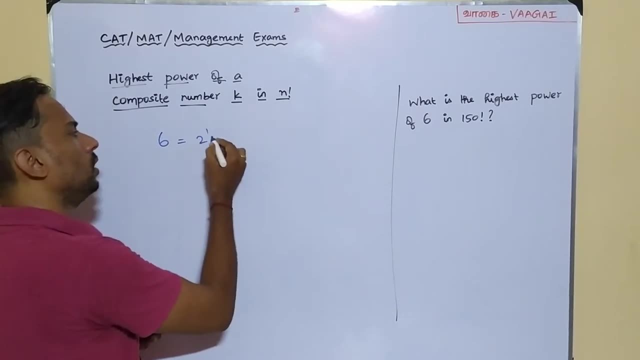 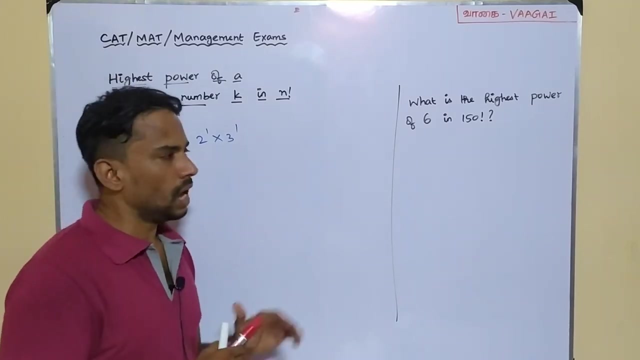 factorial. So in that way, 6 can be factorized as 2 power 1 and 3 power 1.. So this is going to be the factorization, or prime factorization, of our number 6, and we need to find its highest power. 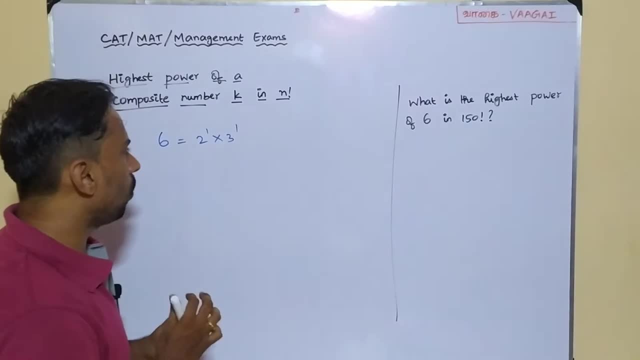 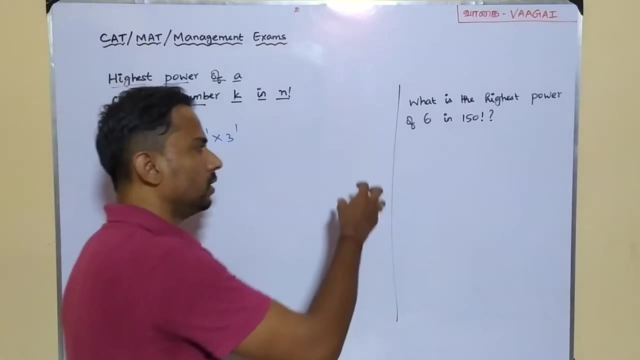 in this 150 factorial. yes, So for that, what we need to do is we cannot directly apply the previous method. How we did that? We took our number, our n factorial, I mean that n value we took there and we did repeated step division. if you remember right, If you have missed that session, 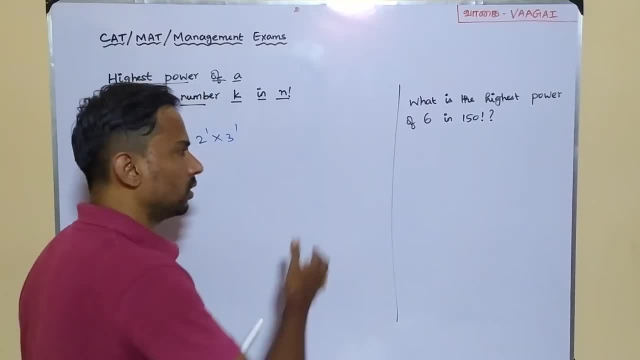 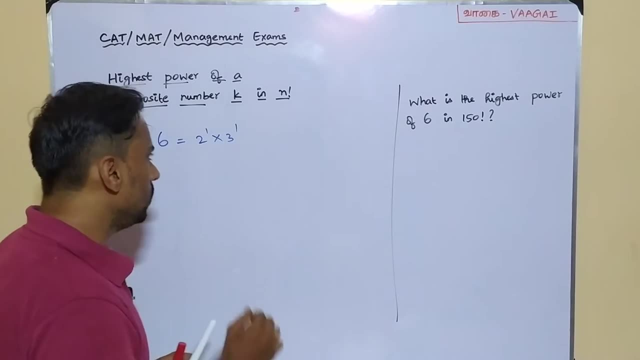 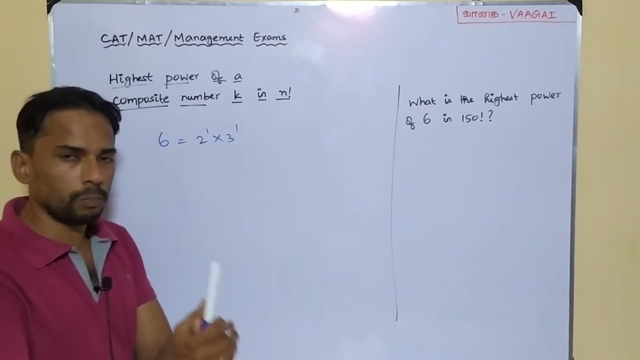 kindly see that video and come here for a better understanding. So there we did repeated step division and from there we got what is the highest power by adding yes. But here we cannot directly employ that method. Why? Because here our number is not a prime number, Here we have got a composite. 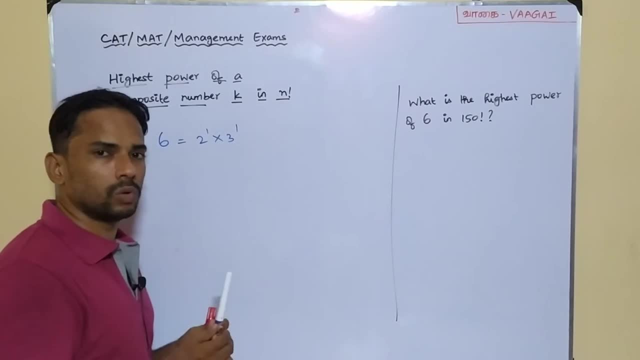 number. That is the reason, right. So in order to do that, we need to find the highest power in that. Then, what we have to do, We have to break our number, and that is what we have done here. yes, 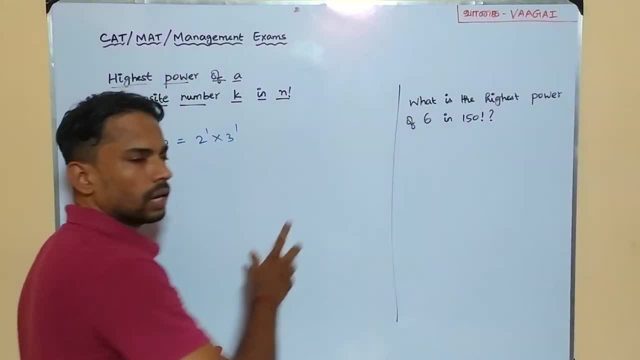 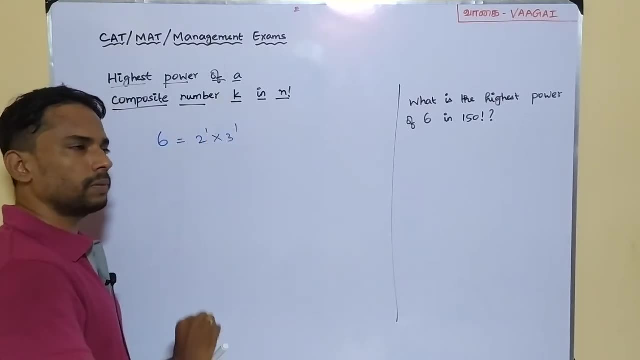 Now, what I am going to do here is, inside this 150 factorial, I am going to check, or I am going to find out what is the maximum power of 2 available and also, at the same time, maximum power of 3 available. Now, these two numbers are prime numbers. Now, very well, I can employ. 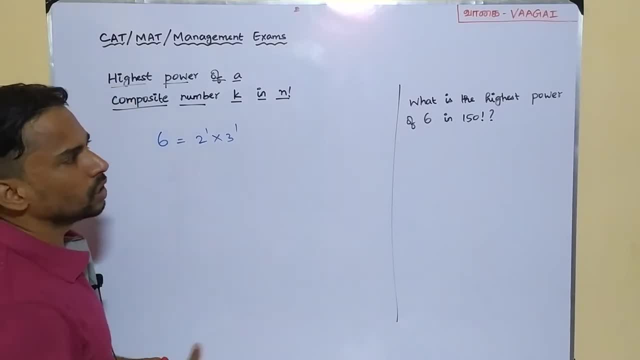 our easy shortcut method right? So let us do that here. So our n value here is 150.. So first I am going to start. So I am going to start by doing it with 2.. That is, I am going to check what is the highest power. 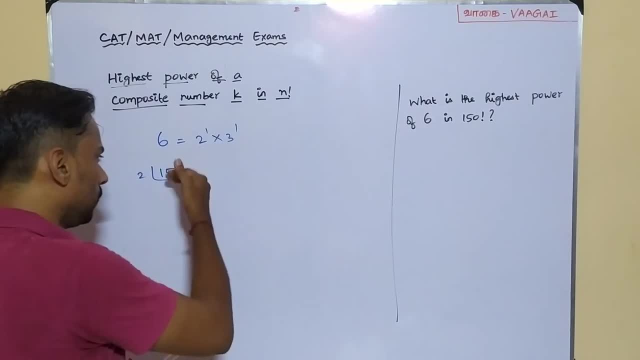 of 2 available in 150 factorial. So let me do the repeated division process. So 150 divided by 2. We have 75 times and once again divided by 2. So we can go up to 37 times. So do it here. 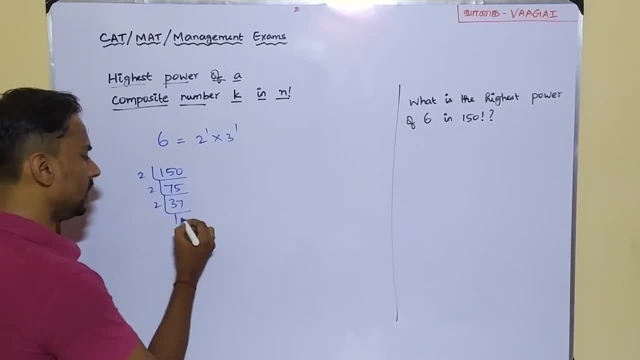 put it here. So once again by 2, we can have 18 times, yes, and once again 18 into. we have got 9 times and 2.. So here this will be actually 4 times and 150 factorial, So we have got 75 times. 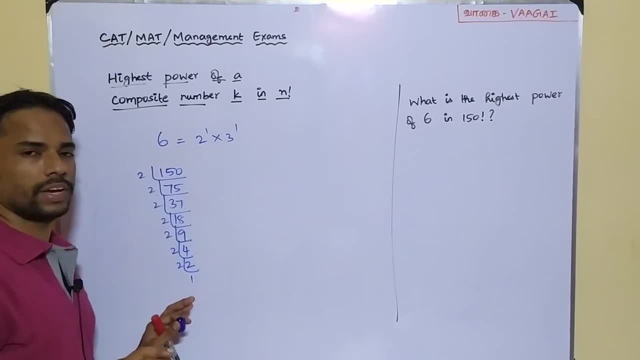 and once again 2, 2 times, and once again 2, 1 time. Yes, we can stop here Further. we can't proceed because we have got a number 1 and this 1 is lesser than this number 2.. So, in that case, stop here. 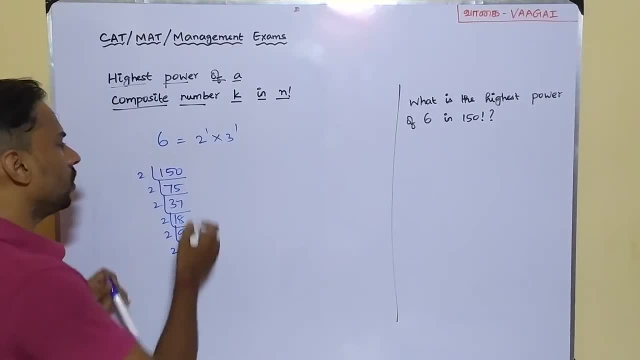 and, as usual, what do we do? We will just strike out our first number, right? We will just separate or we will just eliminate our first number and all the remaining numbers. we will be adding it in order to get the highest power of 2 in this 150 factorial. That is what we usually do, right? 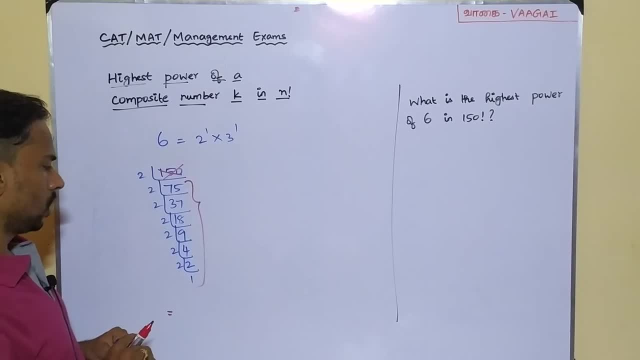 So in that case, what I am going to do is I am going to add all these numbers. So I think we can just add the numbers in sections. So if I try to do it, I will be getting 4 plus 2 plus 1.. This will be a 7, and 7 plus 9 would give you 16.. 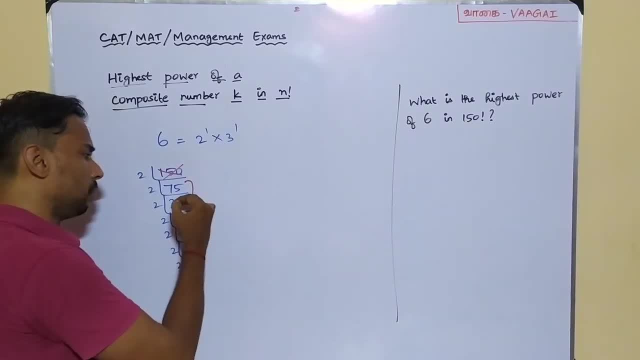 16 plus 18 would give you 34.. 34 plus 37,, 34 plus 37 would give you 71,, I think right. So 34 plus 31 will be 71, and 71 plus 75 will finally give you 146.. 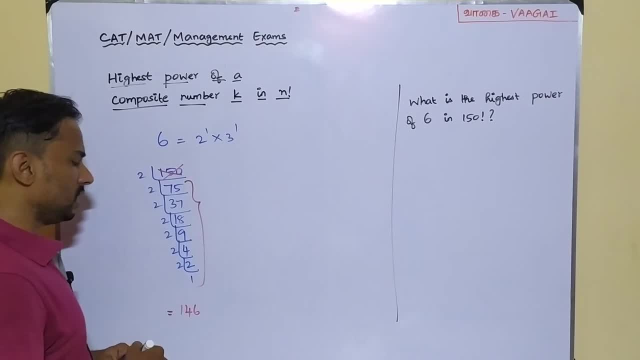 So yeah, you can just check it if you want. So this means I can have 2 power 146 inside this 150 factorial. That is the meaning. okay, Yes, we will have it separately here on the one side, and 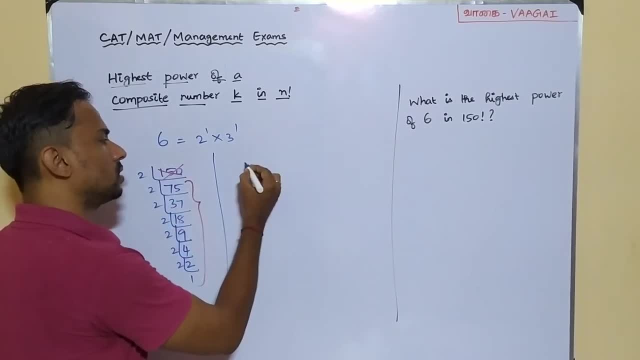 yes, I will just put a line here because I am going to do the same process. I mean, inside this 150 factorial, what is the highest power of 3 available, So for which I have to do my repeated step division process now by the number 3.. Yes, shall we start? 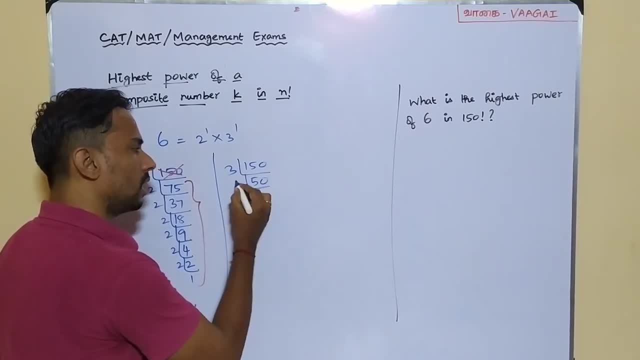 So 150 in 3, it is exactly 50 times, and again 3, I can go up to 3 sixteenths or 48, right, So I can go up to 16 times and once again 3, I have got 5 times because 3 fives are 15, and once again. 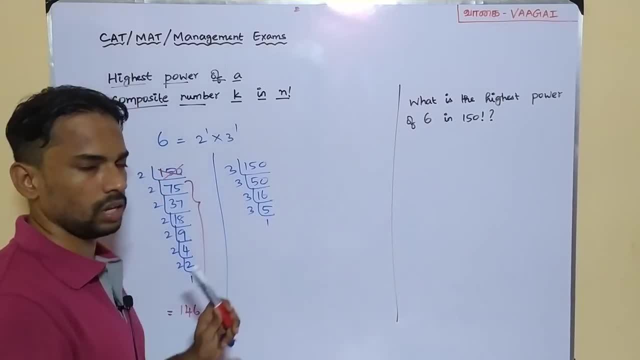 by 3, if I do, I will have only 1 time. Yes, because 3 ones are 3, that is it only 1 time. So further I cannot proceed. Yes, we can stop here. So in that case, now we will be having: 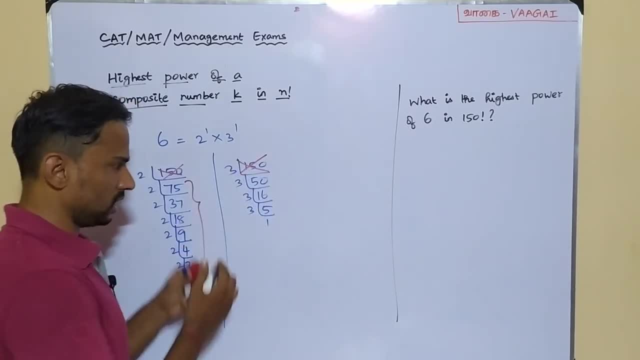 same way, I can just eliminate my first number, 150, from where I started and I can add all the remaining numbers. So this will give me 16 plus 5 plus 1.. This will be giving me 16 plus 5 plus 1 will be 22, and 22 plus this 50, I have to do So. 22 plus 50 will. 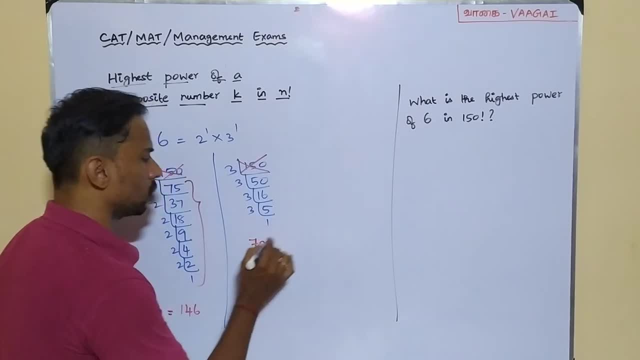 give you 72,, is it or not? So 72.. So this means the highest power of 3 available in 150 factorial will be equal to this 72.. So that means I will have 2 power, 146.. 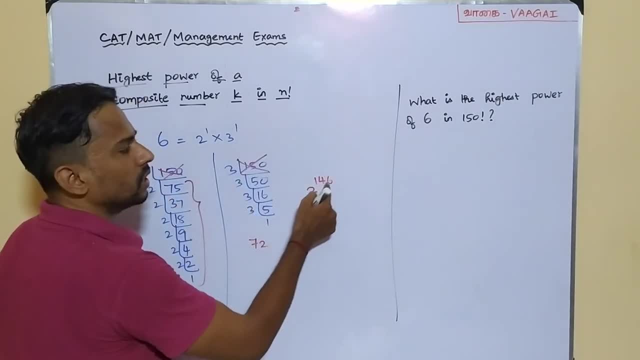 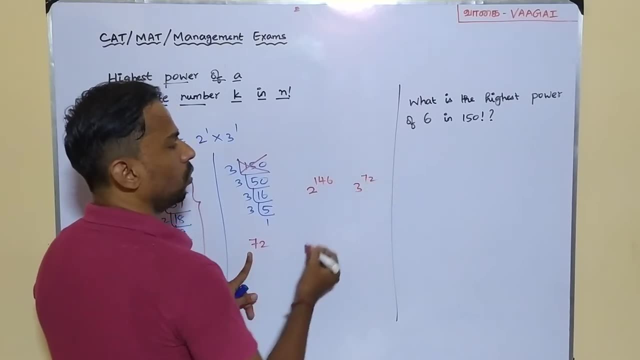 This 150 factorial. So maximum 2s if you have in this 150 factorial, it will be 2 power 146, and same way, maximum power of 3 will be this: 3 power 72. So I can have 2 power 146 and 3 power. 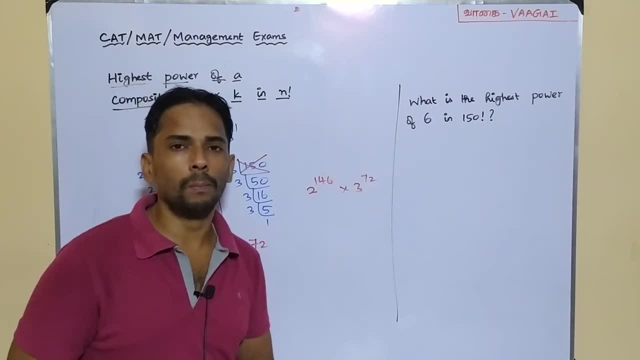 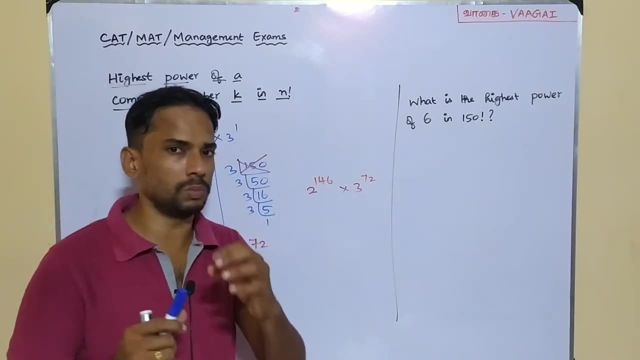 72 inside my 150 factorial. But now what we need? we need the highest power of 6, only right. So in order to form 1- 6, just remember, this point is very much important- In order to form 1- 6,. 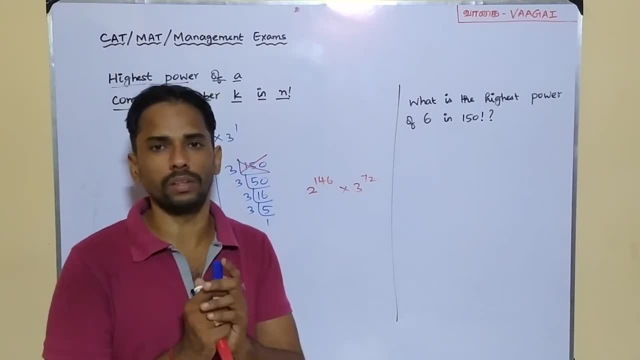 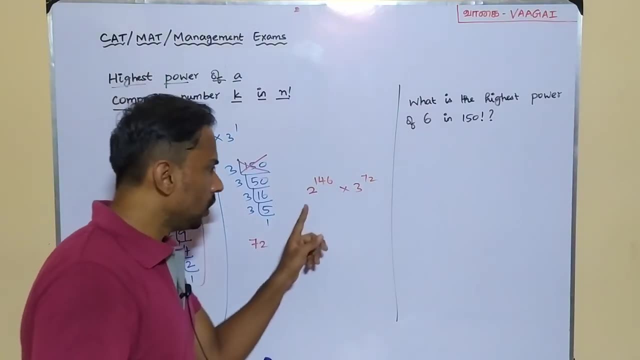 we definitely need to combine 1, 2 and 1, 3 together, is it or not? So 1, 2 and 1, 3, when they merge together, is what will give us 1, 6.. So we have got 146 2s and here 72 3s. So with this collection, with this collection, 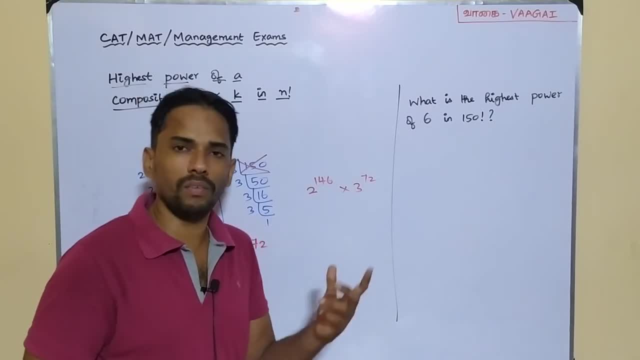 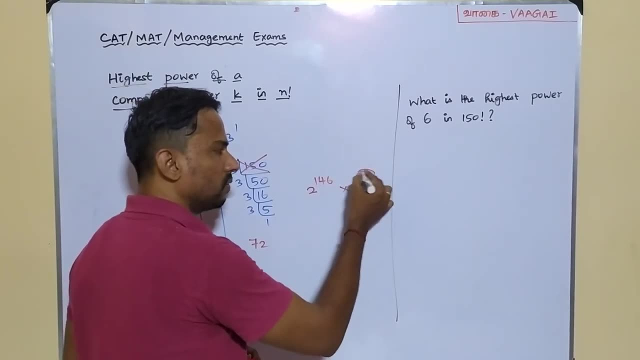 how many maximum number of 6 can we create or can we form That? we have to think. It is very easy for us to understand that here the lesser power, when we compare among these 2, the lesser power is 72. So in that case we can form a maximum of 1, 6. So in that case we can form a. 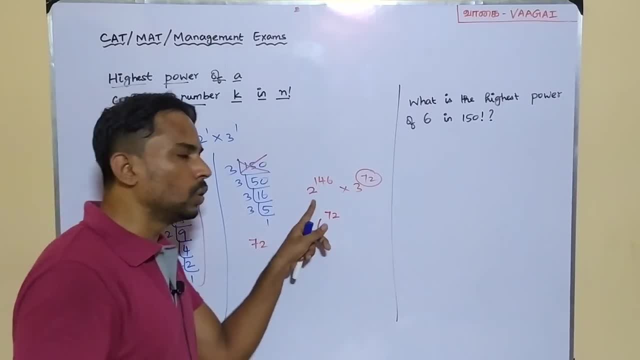 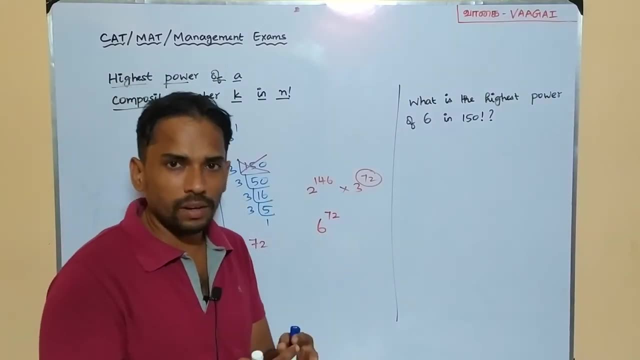 maximum of only 6, power 72. Why? Because the other 2s, I mean the remaining number of 2s- will not have its pair of 3 to get it collide and form a 6. That is the reason. So here we may have still. 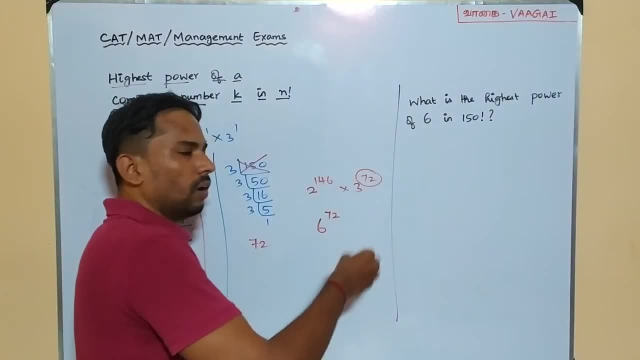 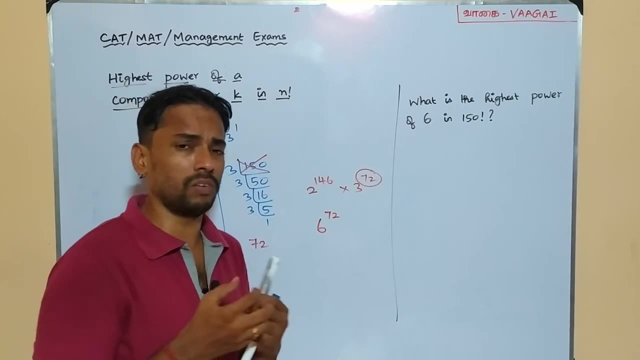 2 power 146, but all these 2s will not have a pair 3. So maximum I can form only 6 power 72. So that means the highest power of 6 available inside this 150 factorial will be equal to 72.. 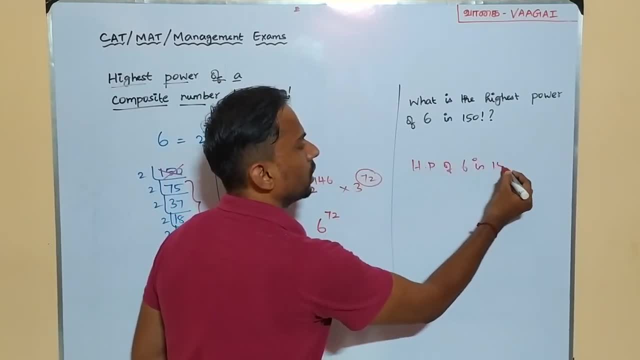 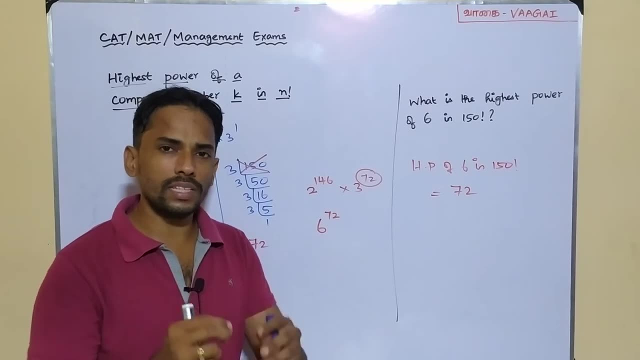 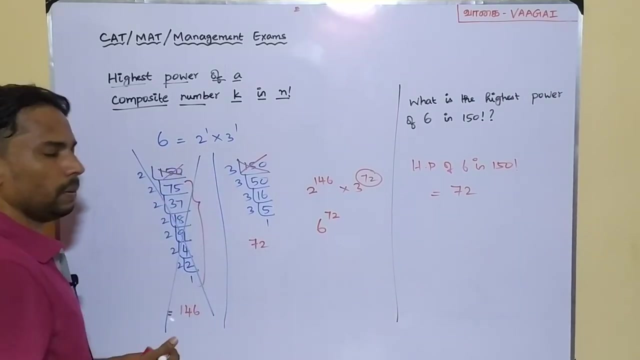 So the highest power of 6 in 150 factorial, the answer would be 72.. And if you are very wise enough, or if you are brilliant, you can easily guess it here itself and you can save your time by not wasting or not doing this calculation. Why? Because here I have to do 2s power and 3s. 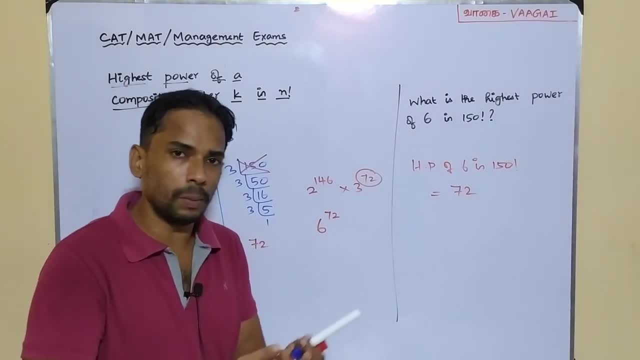 power, If I am able to visualize, or if I am able to realize it in prior, that only the 3s power will be minimum in count. it is not going to be 0. So I am able to visualize, or if I am able to, 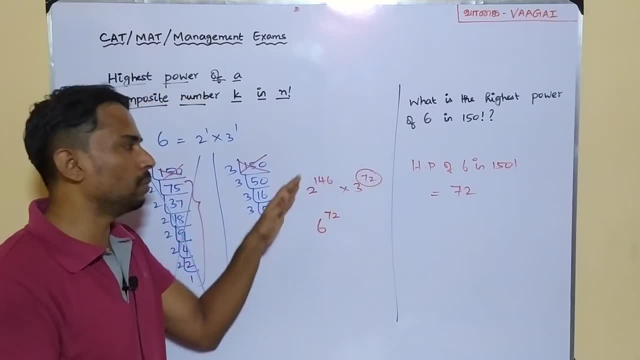 visualize it in prior that only the 3s power will be minimum in count. it is not going to be 0. So this is why it is not necessary for us to just worry about what can be the maximum power of 2.. 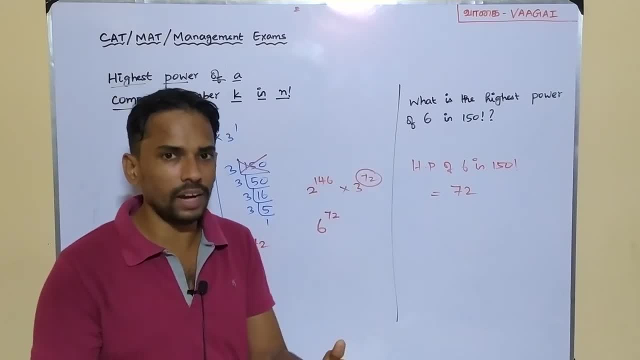 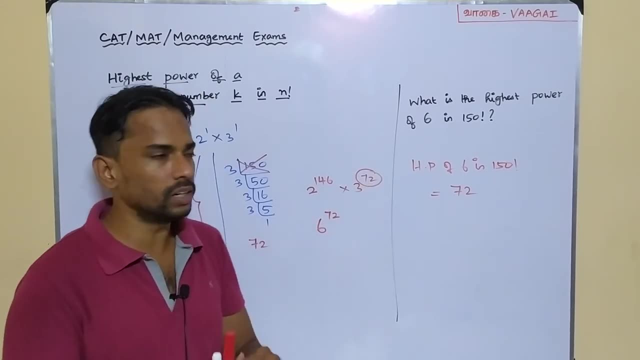 Whatever it is, it will be definitely more than 3s power. So if we realize it at the first itself, so very well, we can save our time. we can just go for directly 3s power. How we can do that is. 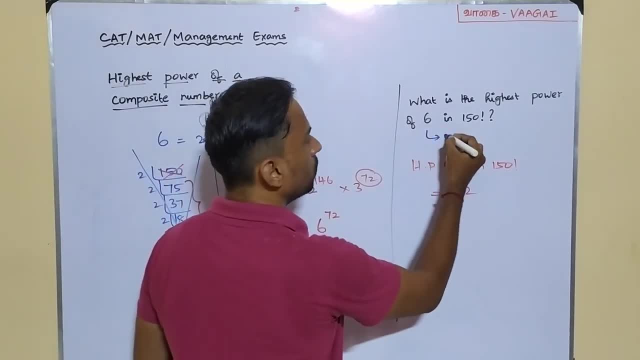 just break this 6.. So when you try to break this 6, you will be getting 2 into 3, right, 2 power 1 into 3 power 1, this is what you will be getting and just go for the highest number, 2 and 3,. 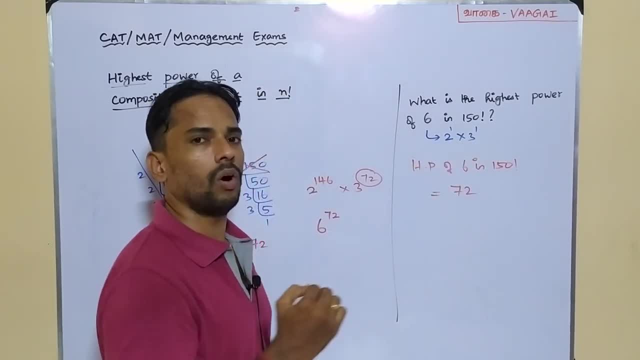 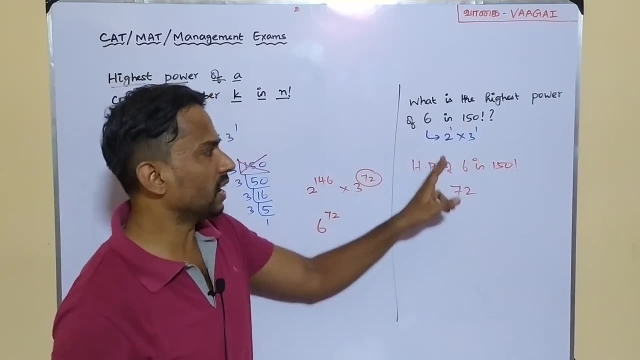 the highest number is 3 and you can directly go test or go find the highest power of that 3 alone, instead of wasting your time in finding what is the highest power of 2.. Obviously, highest power of 2 will be definitely more than highest.